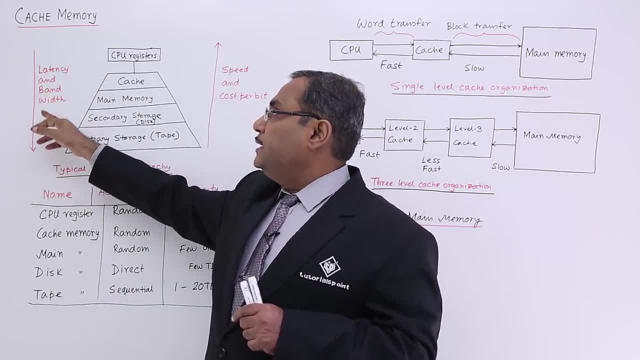 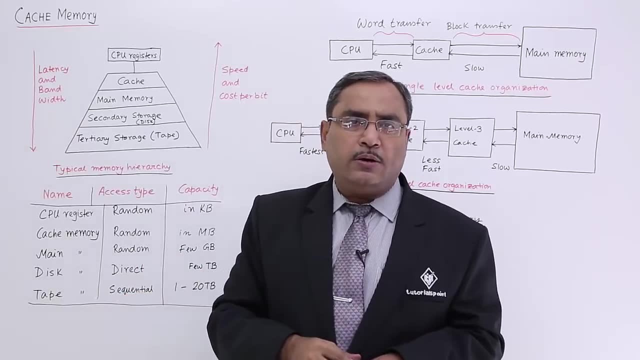 Because in the downward direction, it is increasing. Regarding the latency, what is the meaning of the term latency? Latency means delay And the bandwidth, that is, the amount of data which it can hold, will be. the will be higher in the lower levels. 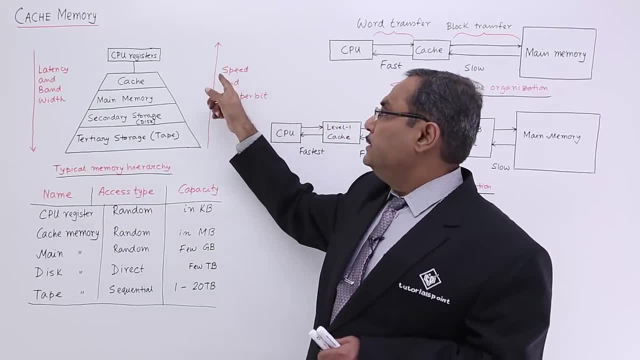 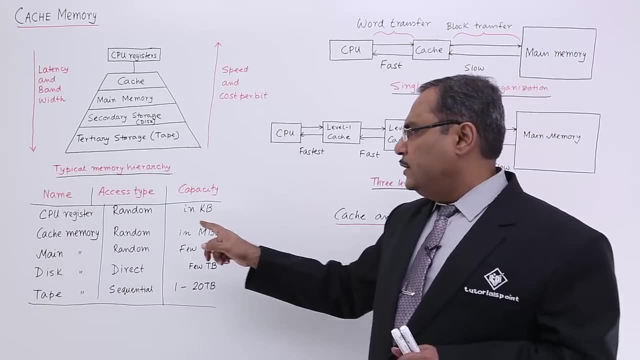 And it will be low. it will be higher in the upper levels. There is a speed and the cost per bit. That is, the speed and the cost per bit is a comparative table, which is which are available here. So here we are having the 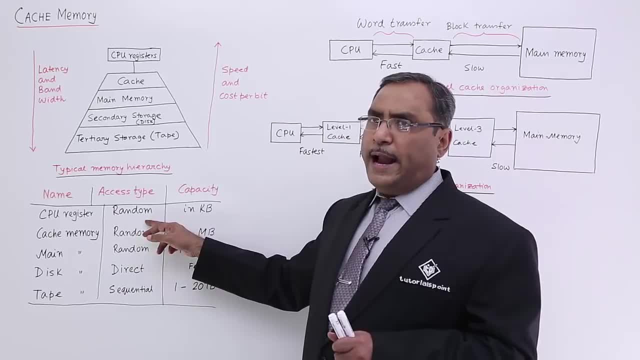 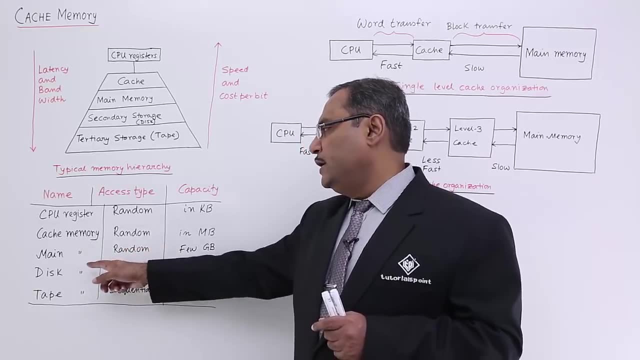 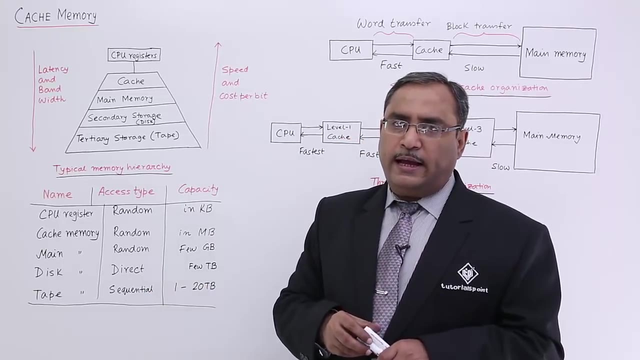 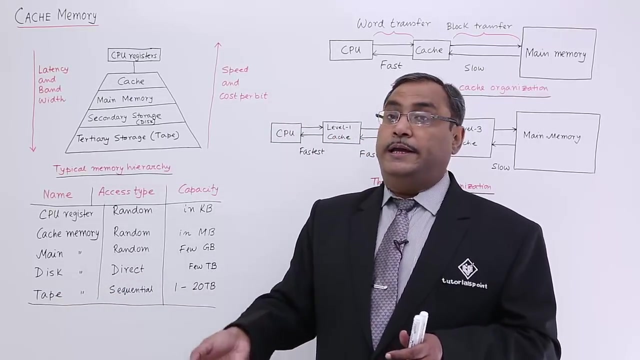 CPU registers which will be accessing access type will be random. you can access any registers at a time. did not go for sequential accessing. cache memory will be also random. main memory is also random. disk memory is direct. you can directly access to that required sector track and the cylinder data and tape memory is sequential. we know that in our audio cassette also in 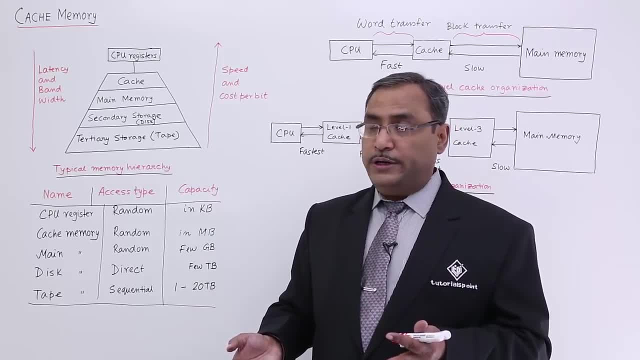 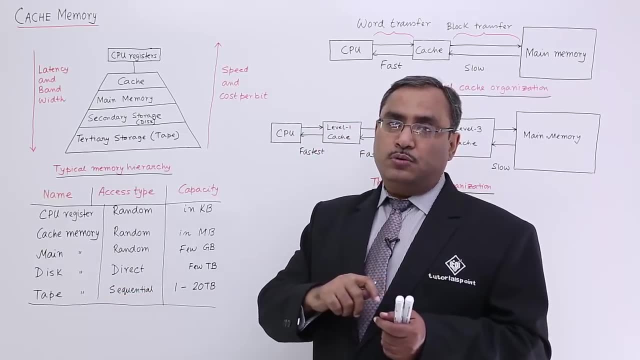 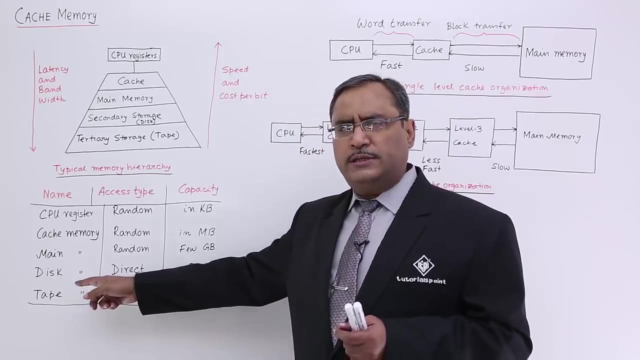 our days. nowadays audio cassette has become almost obsolete. in our days we had this audio cassette there. we found that if you want to listen to the fourth song then you should have to go sequentially. you should bypass first three songs, then you can access the fourth one. So that is. it is a sequential always. tape accessing will be sequential in. 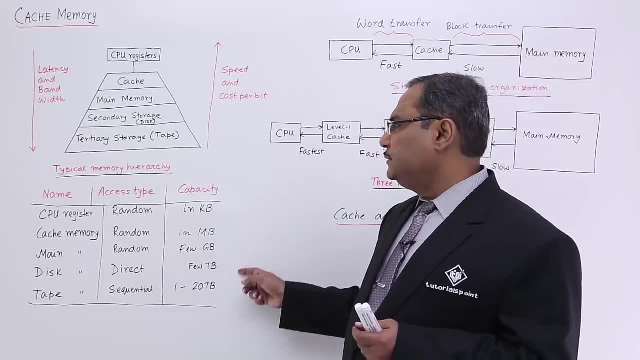 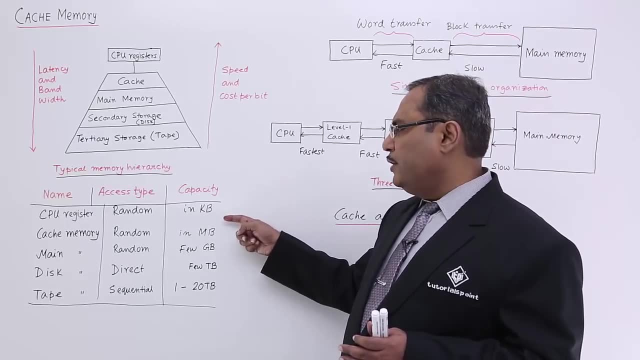 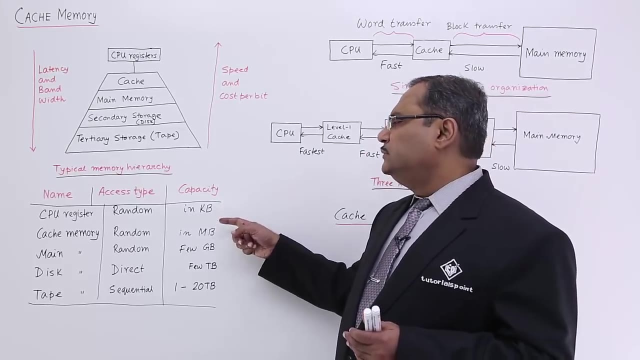 nature. this is the capacity. this is the capacity. So almost it is common that always will be going for 1000 times. always it is going for 1000 times. So the CPU registers will be in the form, in the terms of KB, sometimes for the very 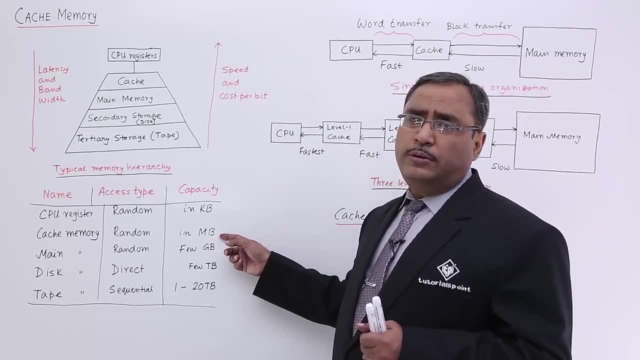 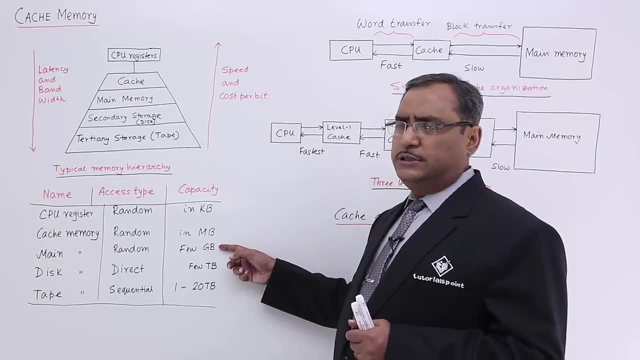 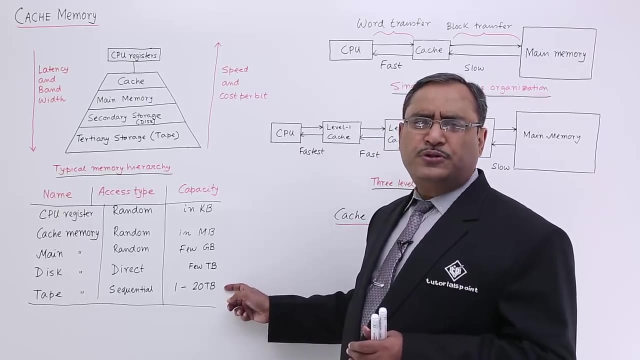 high end it might be MB, and cache memory is now in MB. in the higher range range it is also going to GB, and then we are having this main memory, which is nowadays in GB, and we are having the disk storage, which is nowadays in TB, and this is the tape has become obsolete. 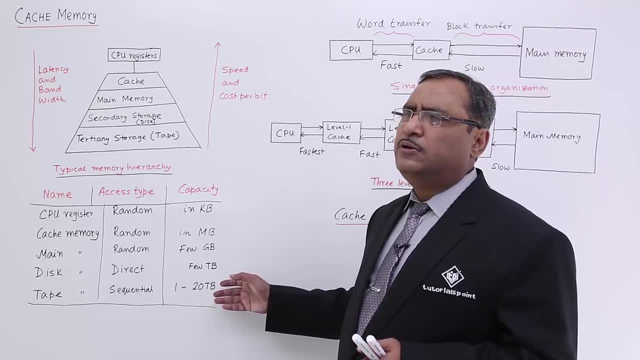 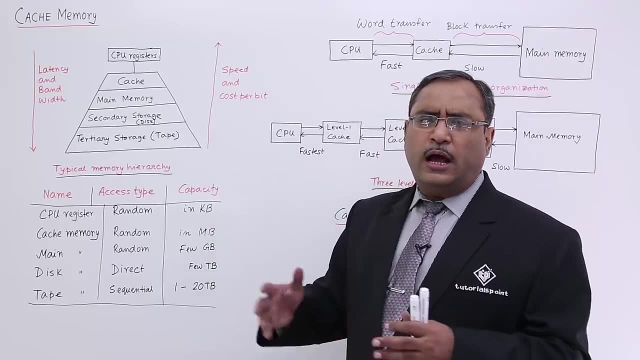 So that is why it is. I found that it is. it was having a very fast memory and this is having 20 TB around. it is having the size. So obviously this sizes may differ, because that will. that will also along with the, along with the progress of time, the sizes will be. 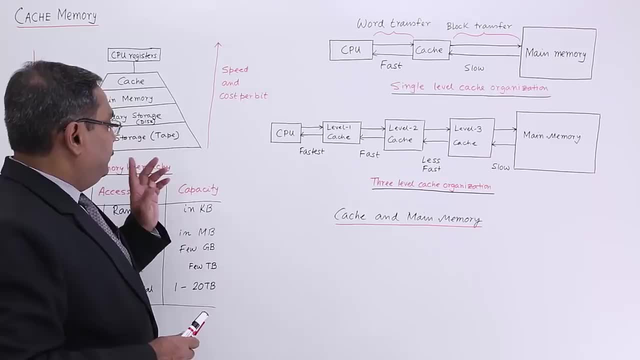 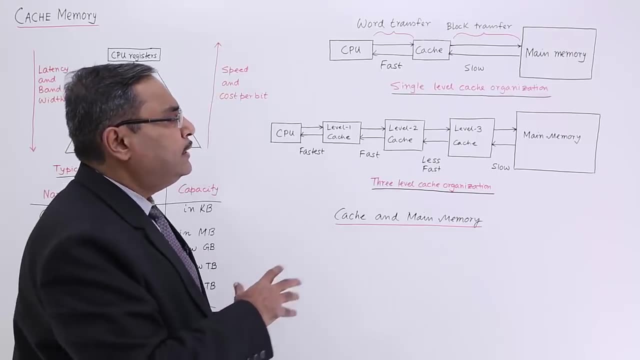 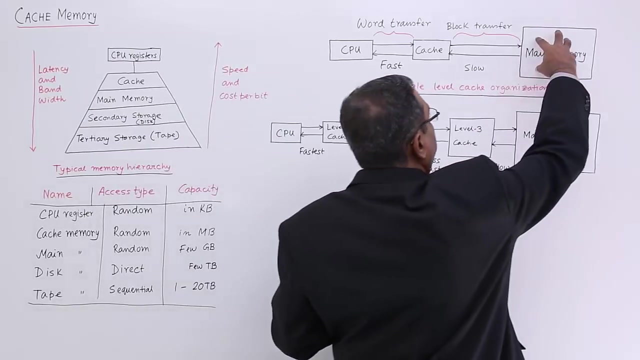 also increasing in the in the case. ok, did that. Now the thing is that where this cache is actually, where this cache is there, we know that whenever a program executes, always the program has to be loaded on to the computers memory, So that is the main memory or the. 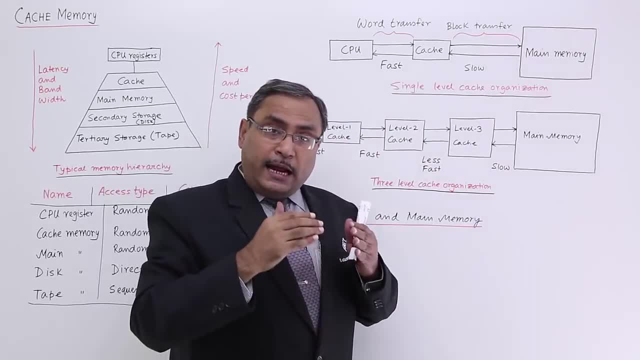 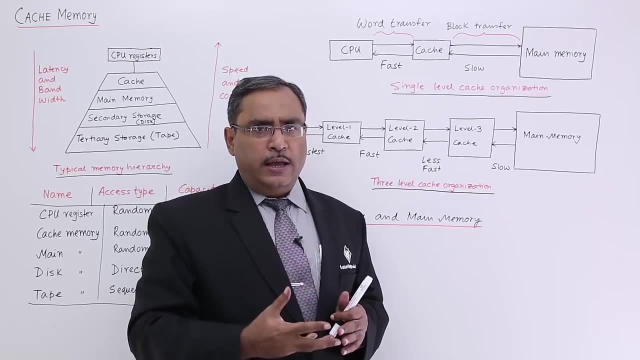 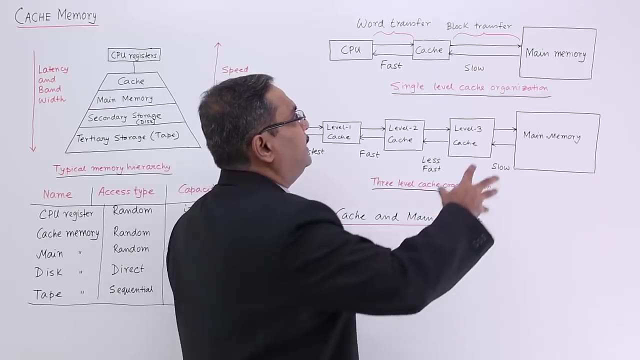 RAM Where the program is getting loaded, and that portion of the program which is very much executing very frequently, which is executing very frequently and which is the most probable portion of the program is going to be executed next in near future. we shall keep them in the cache memory. So cache memory to CPU data transfer will be the faster compared. 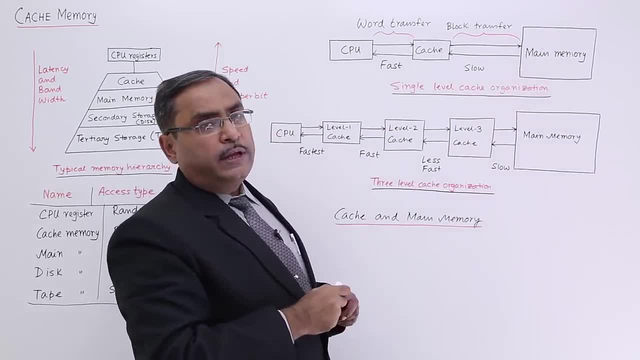 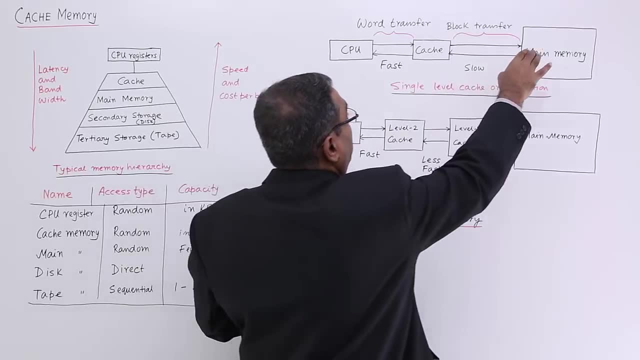 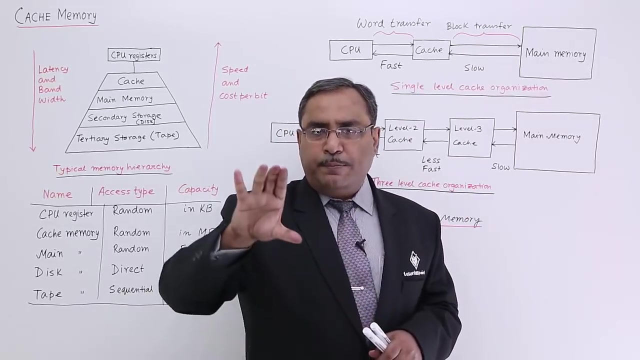 to the main memory to cache memory. data transfer From the cache memory to the CPU, the. the data will be going in forms of words and from the main memory to the cache memory it will be coming in the form of block or in the form of page. it will come. That is the bulk of. 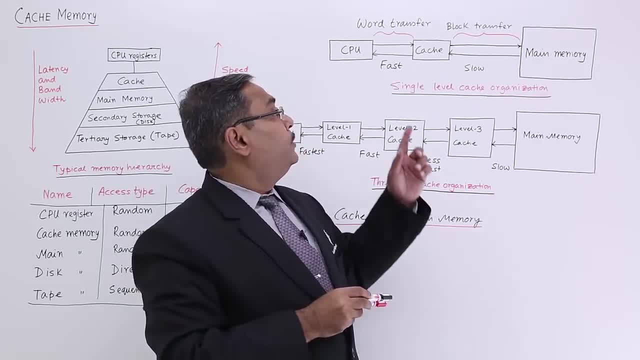 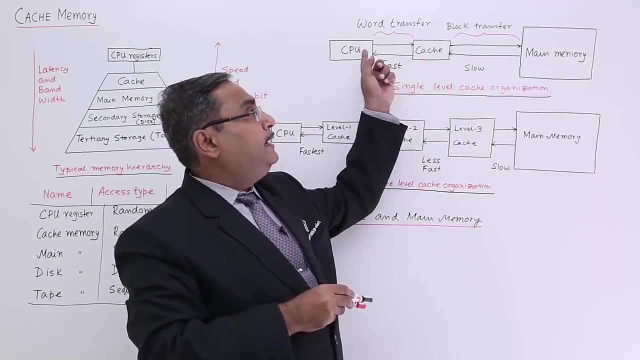 information will be coming from main memory to the cache memory. So this is known as single level cache organization, because I am having this cache only in one level and in this way it will. it will be done Here. the cache box size- rectangular size- is lesser. 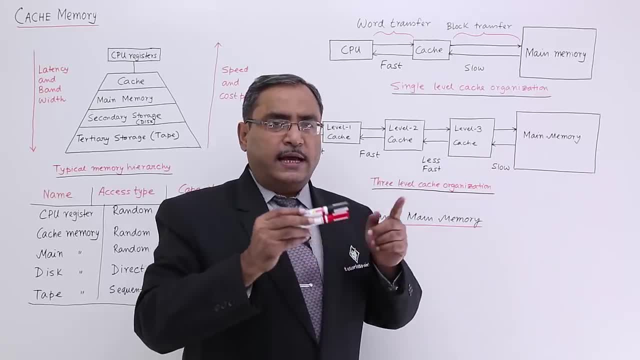 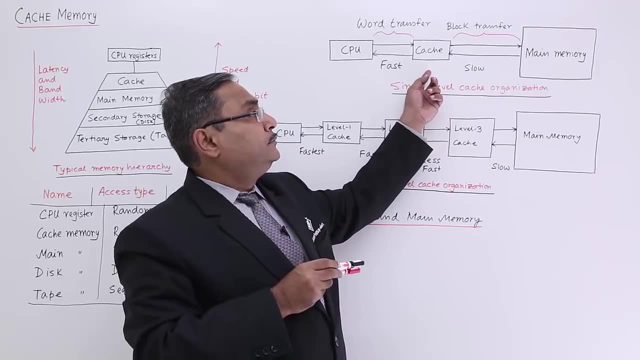 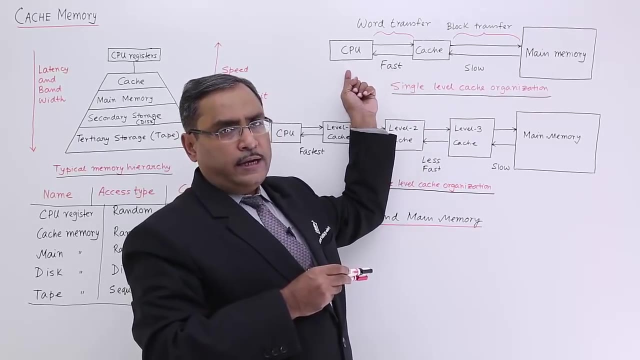 compared to the main memory. You know the reason: because cache size is lesser than the main memory size. So that is why I made that one symbolic here in this particular diagram. Now what will happen? let us suppose CPU is trying to access one instruction, the instruction or data, If the 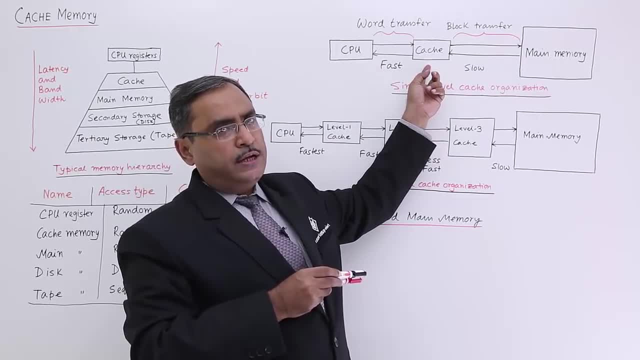 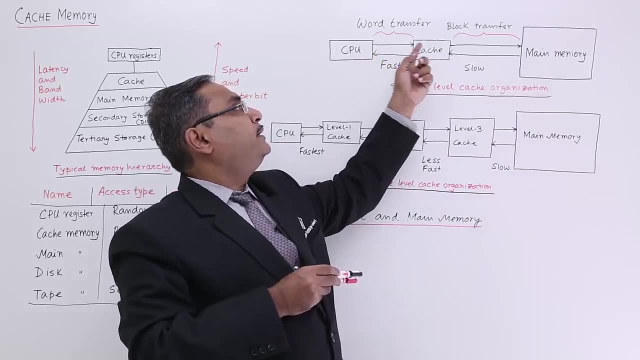 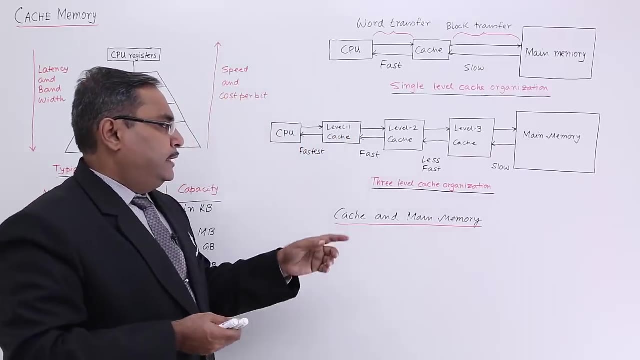 data has been found in the cache. that is known as cache hit. If the data has not been found, then it has to be mapped from the main memory to the cache memory and then that corresponding data or instruction will be Mapped by the CPU or will be accessed by the CPU. There is another kind of organization. you can consider for the cache. There is a multi level cache organization. We are having this L1 cache. level 1 cache can also be called as L1 cache. We are having this L1 cache. its size is smaller to compared to L2 cache and L2 cache is having the size smaller to L3. 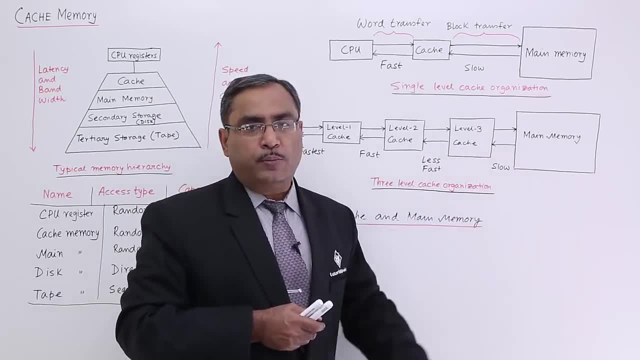 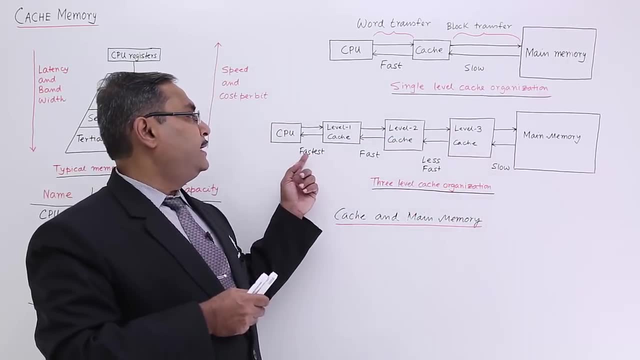 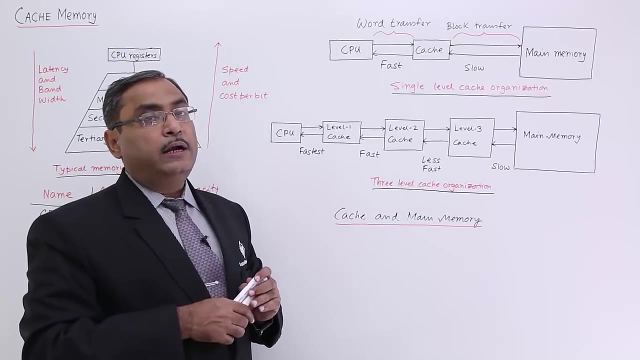 cache and L3 cache is having the size smaller to main memory. So that is why the recognition, the incredible, a rectangle sizes area. So here the accessing time is fastest, here it is fast, less fast and it is slow. So also a cache memory may occur in multiple levels. 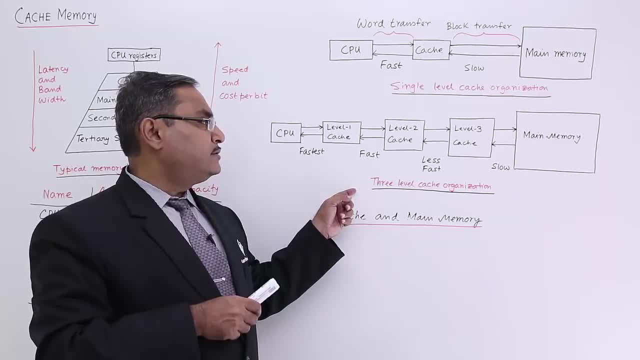 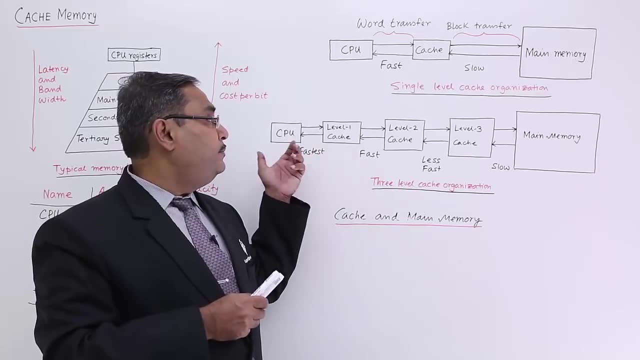 So level 1, level 2, level 3 in this way and that is known as 3 level cache organization, or also you can call it as multi level cache organization. So cache memory is residing in between the CPU and the main memory in this particular fashion. So that is a first.